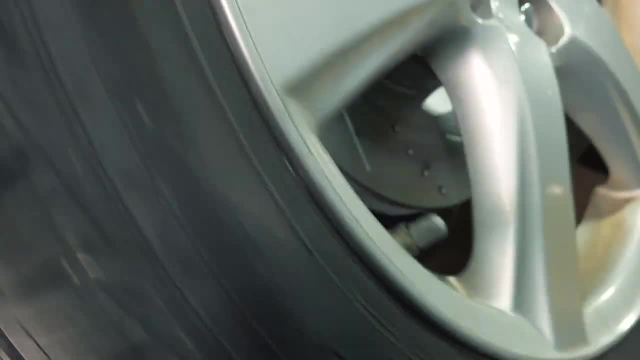 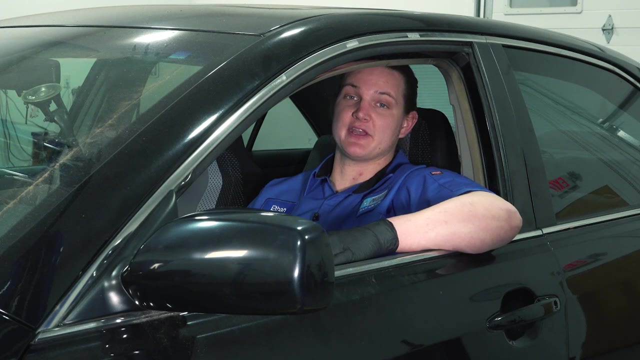 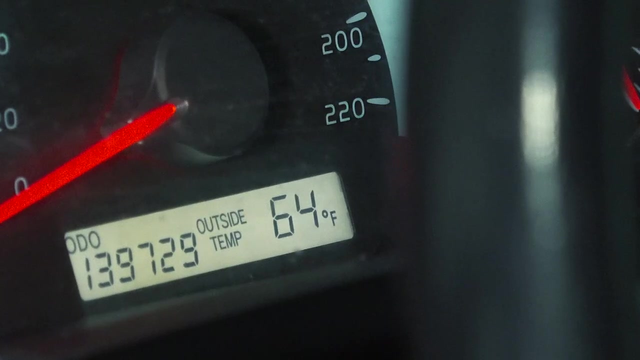 an automatic transmission may experience a hesitation when accelerating. A software update for the onboard computer may be available. This update should help to clear up any hesitation in the transmission. This is most common on newer cars. On higher mileage cars, worn components could cause the same hesitation. This would include parts like a torque converter or a. 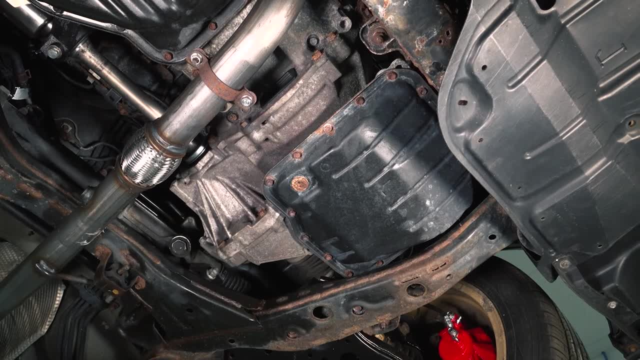 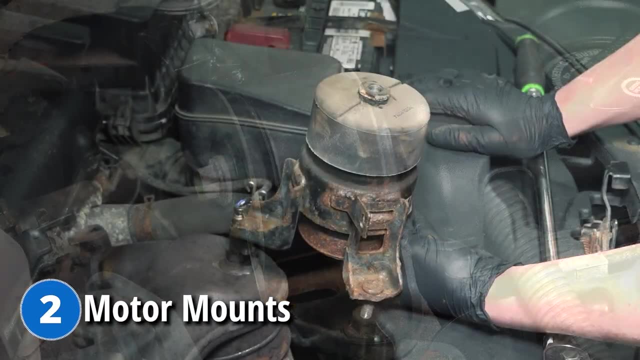 clutch pack. If these parts need to be replaced, the transmission should be updated as well at the time of repair. Problem number two on our Toyota Camry is going to be the motor mounts. The motor mounts at higher mileage may wear out, causing extra. 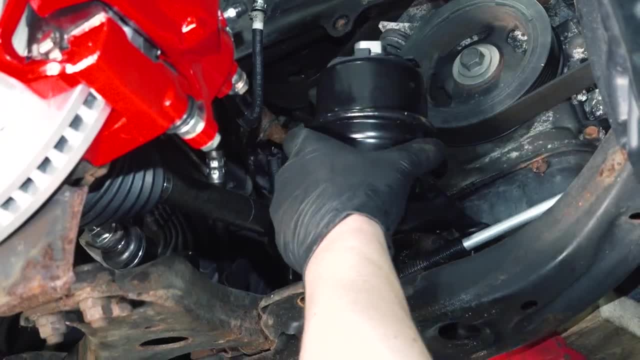 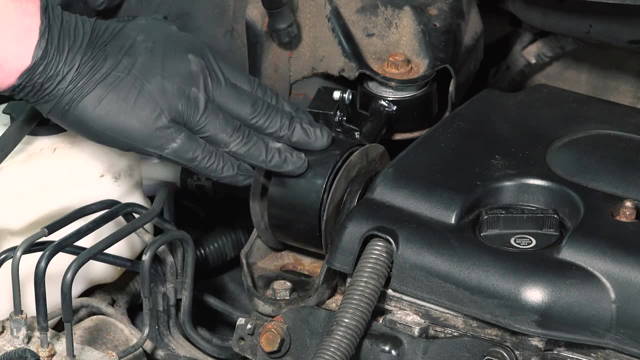 stress on other motor mounts. It's best to replace these motor mounts as they go so you don't put excessive wear on any other motor mount. On these Camrys, we've found that this top motor mount is the most common one to go, which is good for us, just because 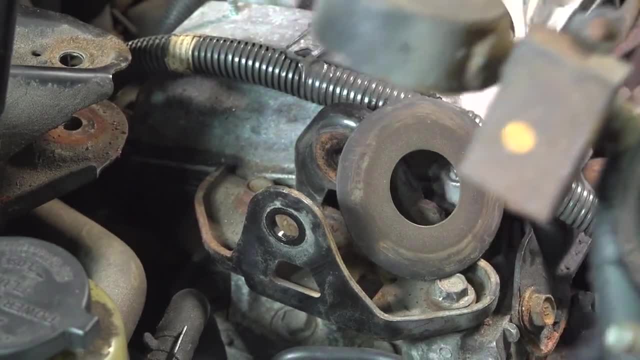 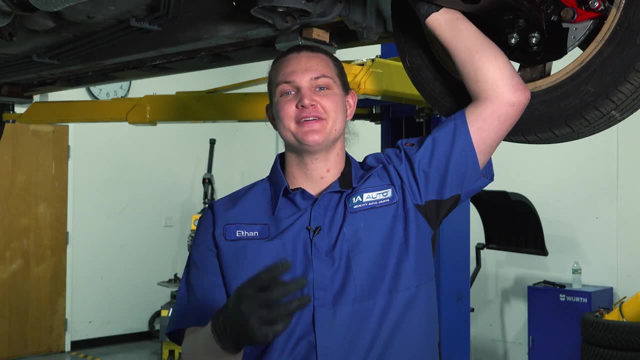 it's two bolts. You can pull it right out, put the new one in and you're good to go. If you need this part or any other part, check us out at 1aautocom. Problem number three on this Toyota Camry is that it doesn't have an automatic transmission. You don't have. 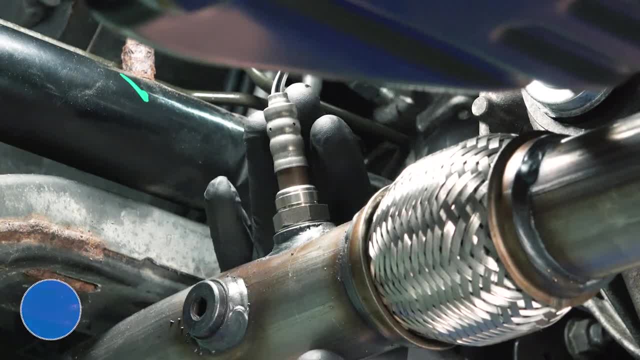 to worry about that. You can just pull it out and it's good to go. Problem number four on this Toyota Camry is going to be our rear O2 sensor. When this rear O2 sensor goes bad, it's going to trigger a P0138 code. You're not going to notice any. 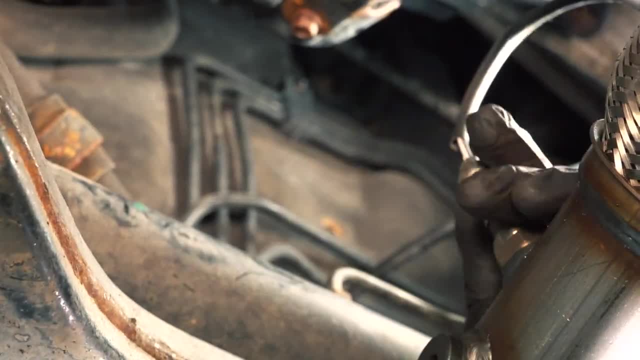 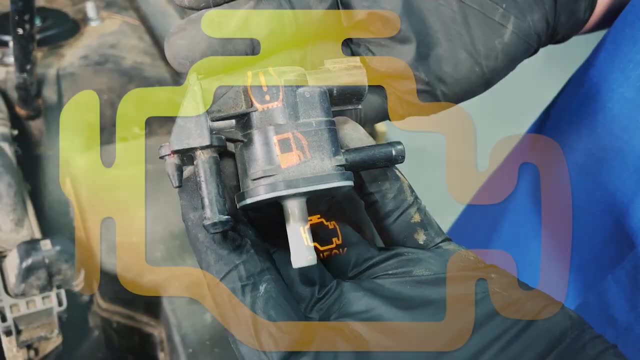 symptoms when driving. You're just going to get a check engine light. Problem number four on this Toyota Camry is going to be our purge valve. A faulty purge valve will cause the check engine light to illuminate in the car. This is an easy fix. All you'll need to do. 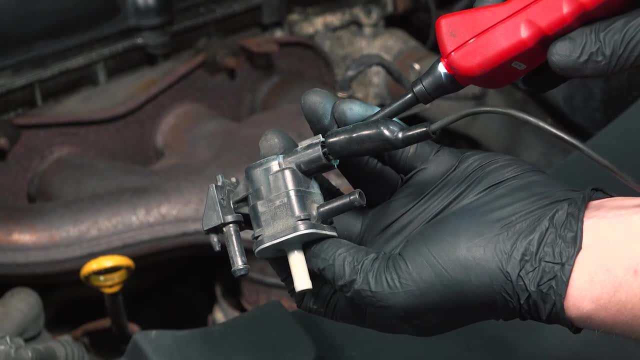 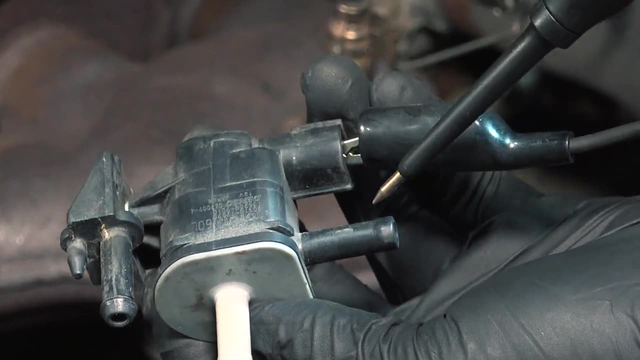 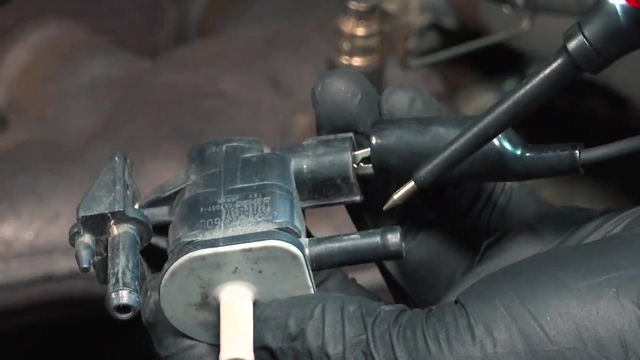 is switch out the purge valve. This is the valve in the engine compartment Inside of the purge valve, opening and closing So air is able to go in and out. when it's given power or it loses power, Then the valve shuts off and now you cannot push air back. 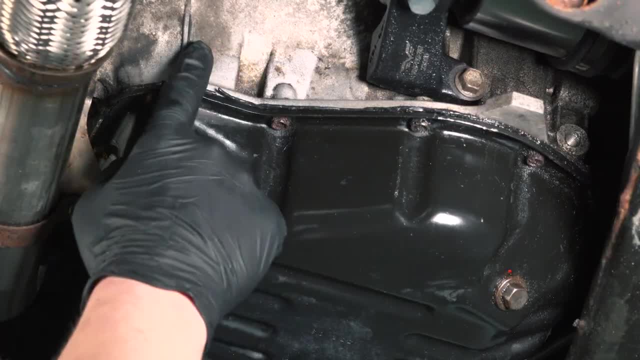 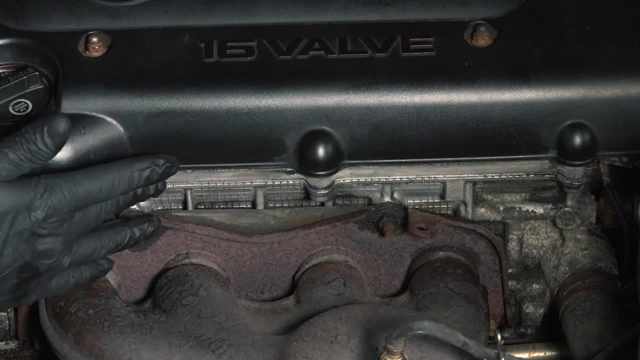 through. There's no oil leaking from the head gasket- The oil pan's good too. There's no oil coming out of the valve cover, And that's going to bring us to our final problem on this Toyota Camry: Excessive engine oil consumption. Oil consumption on this 2.4 liter motor from. 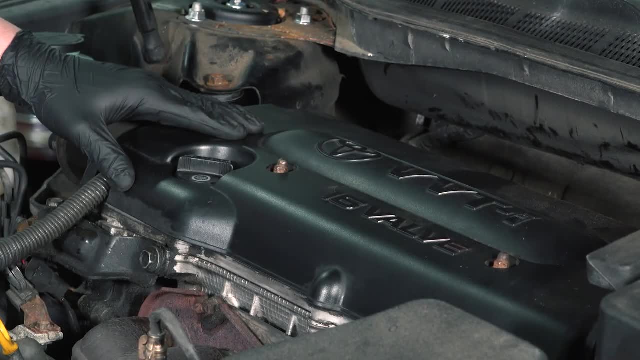 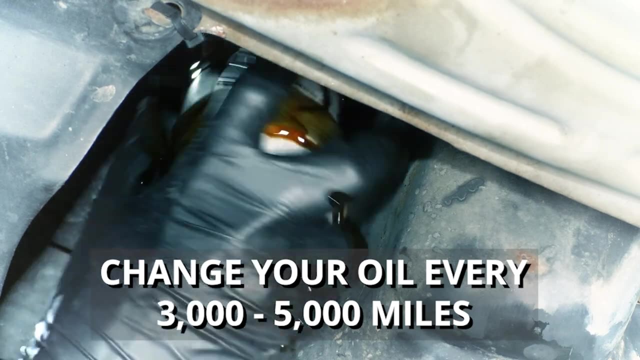 Toyota is a big problem. Other than replacing the piston assembly, we found the best way to combat this issue is to replace your oil every three to five thousand miles, instead of the factory recommended 10,000 miles. If you're in need of an oil change, check us out at 1aautocom.